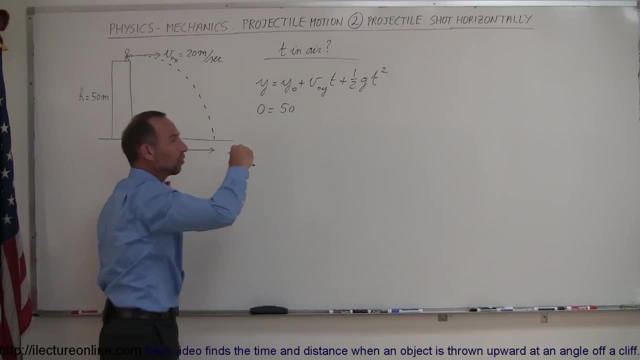 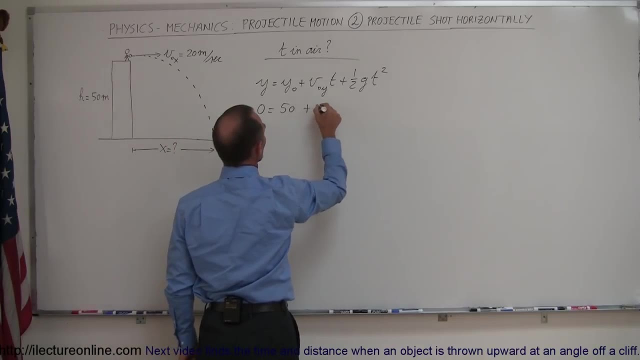 and easier to work with. Our initial velocity in the y direction is zero, because we do not throw it downward or upward, we simply throw it straight out. so it has no initial velocity in the y direction. so this is plus zero, And then, of course, one half times g, since 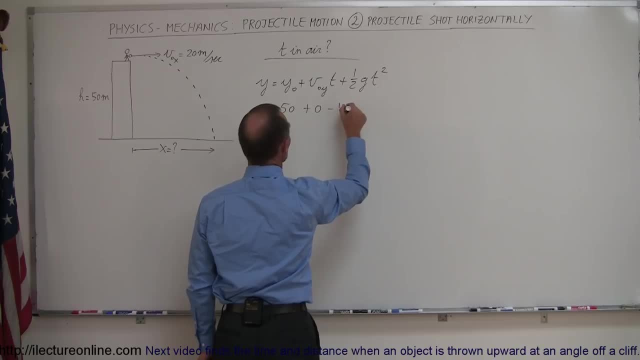 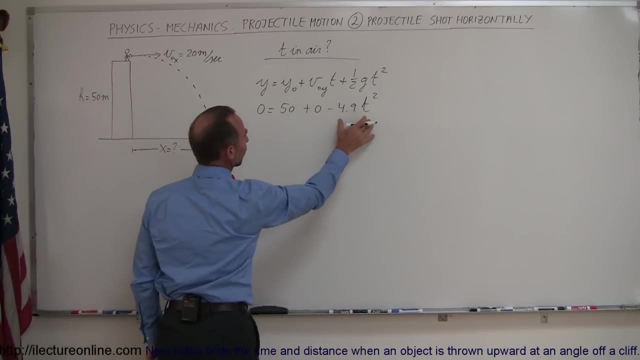 g is a minus 9.8 meters per second squared. this is minus 4.9 times t squared, And we solve this equation for time. Notice, if I move this term to the other side, it becomes positive. so 4.9 t squared equals 50, divide both sides by 4.9, and we get t squared equals. 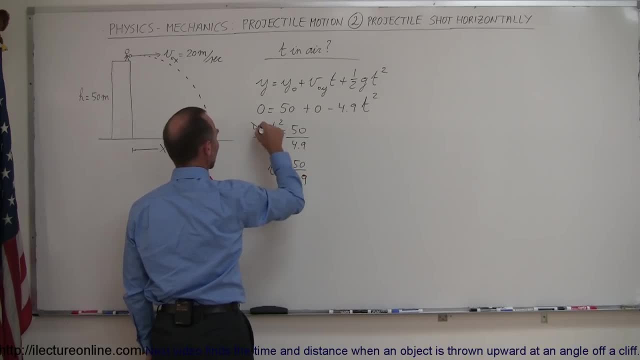 50 divided by 4.9, because here the 4.9's cancel out, and of course then we take the square root and we get 50 divided by 4.9, and of course the units will be seconds and 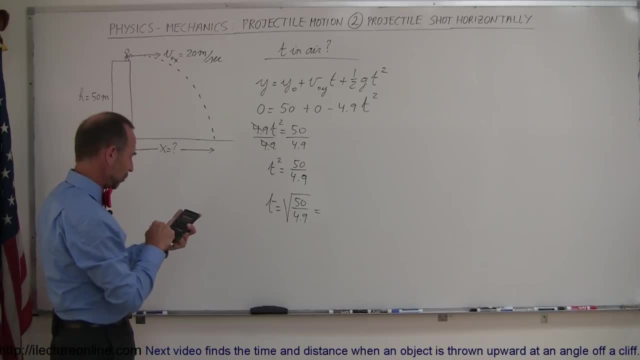 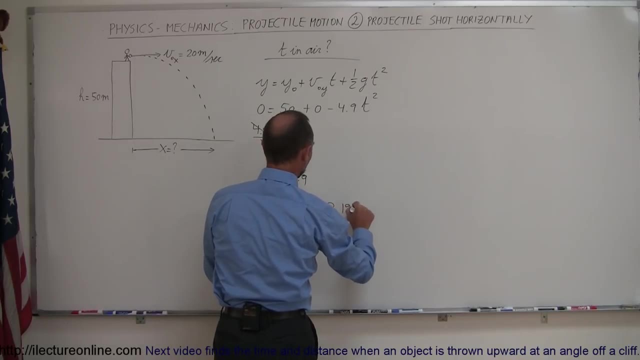 of course I need my time, My calculator for that. so 50 divided by 4.9, and then we take the square root and it looks like it is 3.194 seconds. Now of course I added a few extra numbers, significant figures. 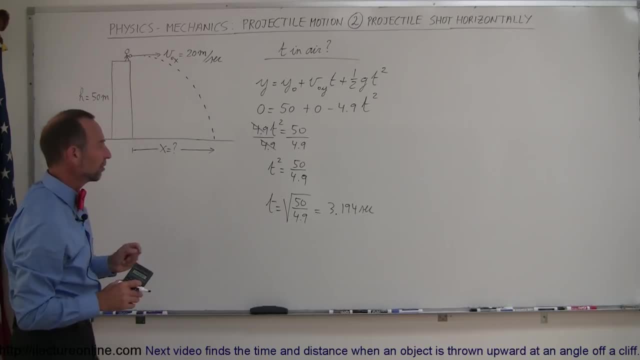 that are not really significant, because I only had numbers to two significant figures, so this prevents me from getting a round off error on an intermediate calculation. So secondly, now we need to figure out how far the object travels. so now we need the very same equation. 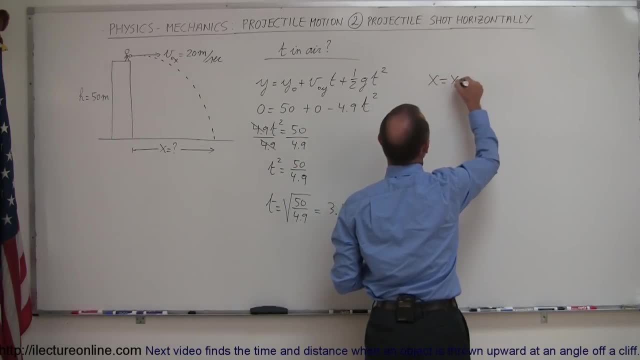 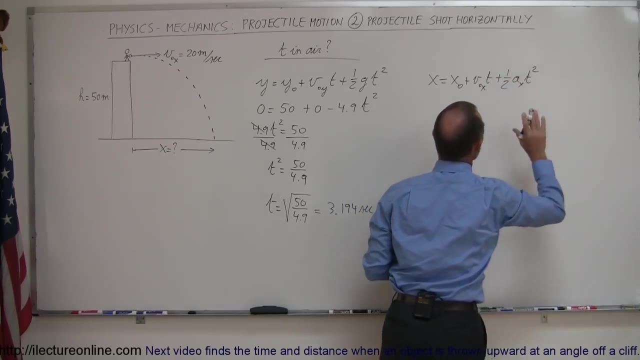 as this in the x direction. So I have x. x is equal to x sub naught plus v sub naught in the x direction times time plus one half a in the x direction times t squared. Now notice, in this case, since we assume x sub. 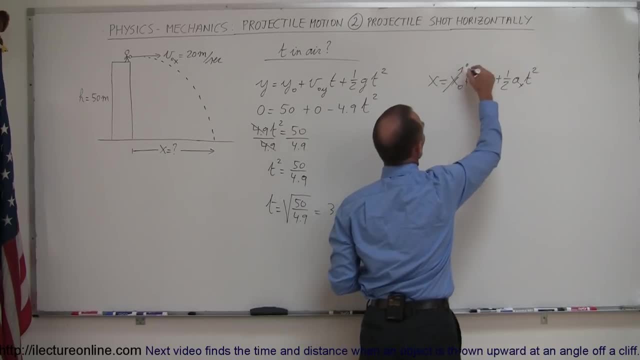 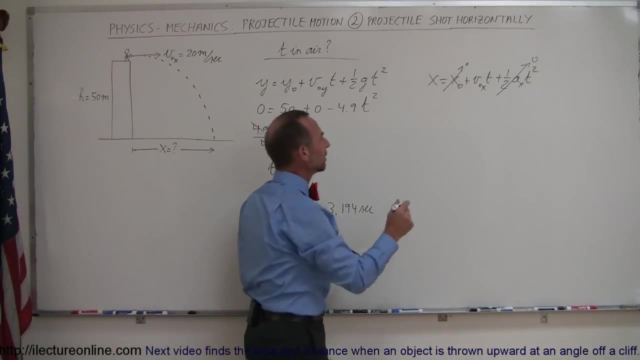 naught to be right here. at the starting point, we can call this zero, and since there's no acceleration in the x direction, because no force is acting in the x direction, that goes to zero as well, and we simply get the equation that distance x equals velocity times time. 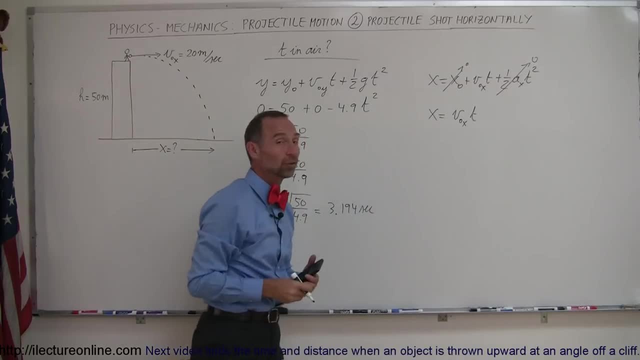 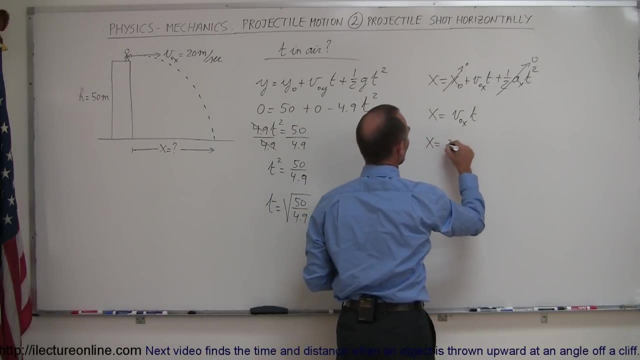 so that's where this equation simply is derived from that original equation. So all we need to know is the original velocity in the x direction, the time which we calculated here and we can figure out the distance. x is equal to 20 meters per second times 3.194 seconds.